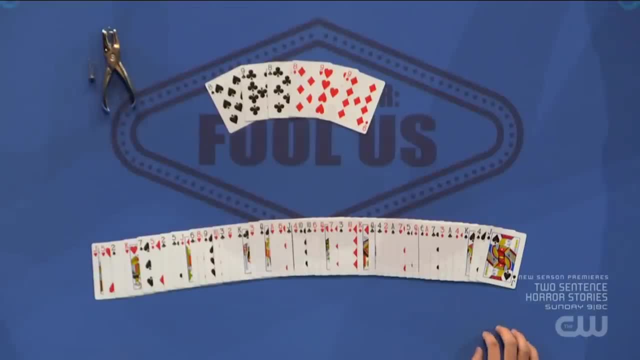 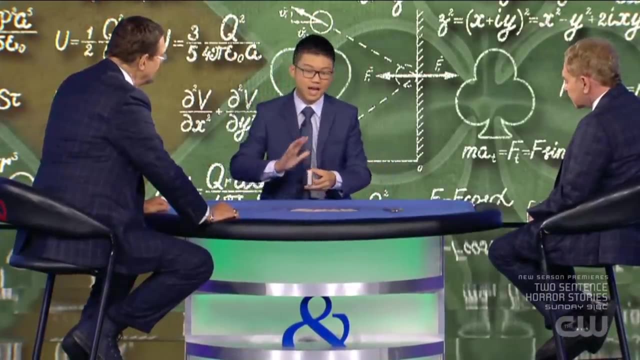 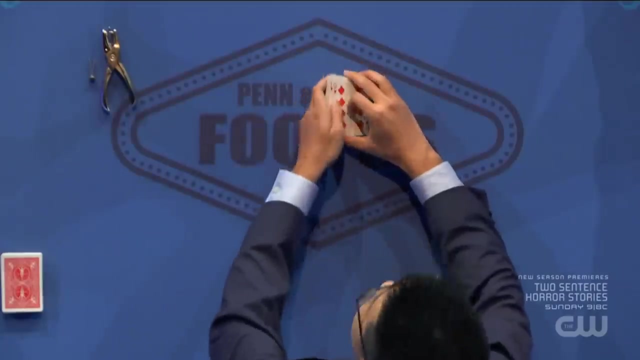 I want you to notice that the rest of the deck is well-mixed. yes, Yes, Perfect. This deck will be our scientific control group. I'll set it aside for now and I won't touch it Now. my research has shown that black ink weighs more than red ink. 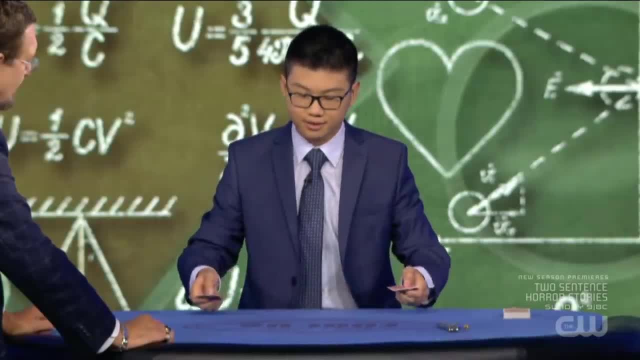 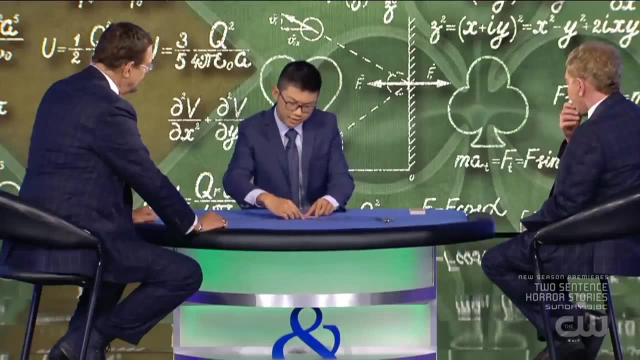 To demonstrate this, I'll separate the cards- three blacks, three reds- and I'll mix them up, alternating: black red, black red, black red. If I pick them up and drop them, the heavier black ink will cause the black cards to pass through the red cards. 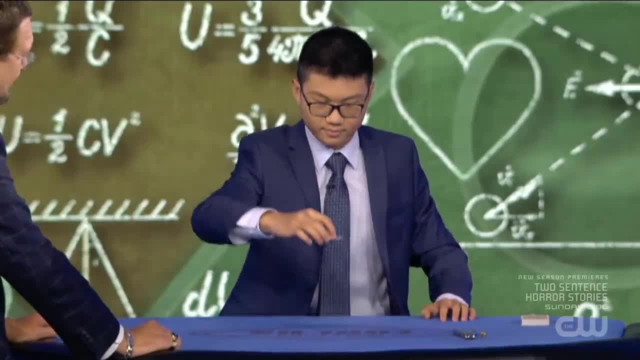 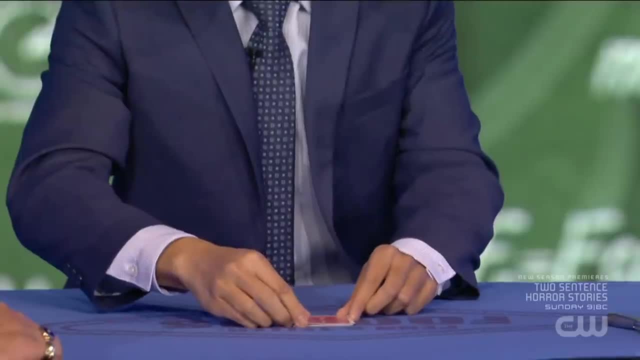 and end up on the bottom. Let me show you There. I think that did it. If we take a look now, the first card, That's a red card. The second card: it used to be a black card, but since we dropped them, 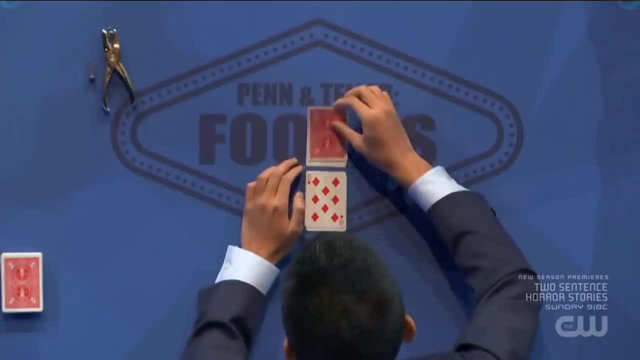 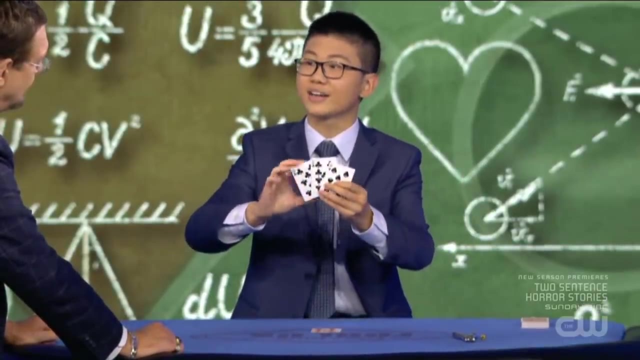 it's also a red card, And the third card, Another red card. Thank you. And if you're wondering, over here are the three black cards, Thank you. Now, I don't know about you, but that seemed pretty fair to me. 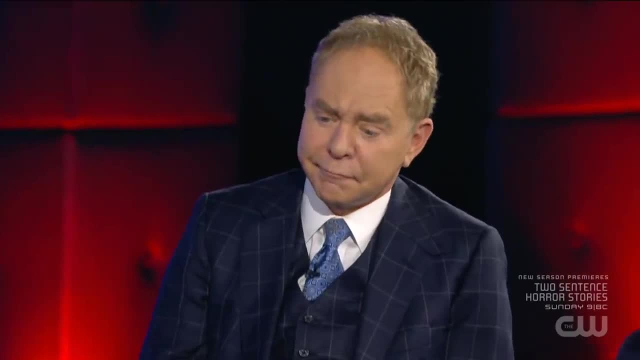 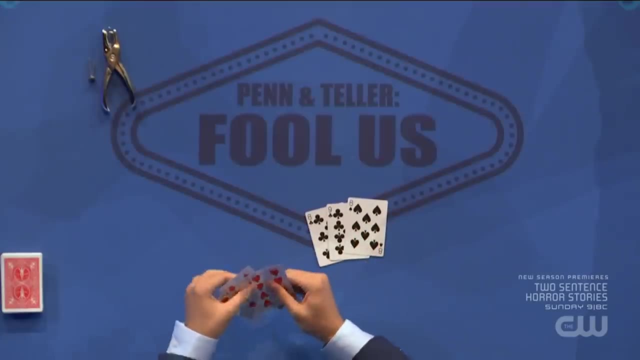 However, I still sense some skepticism, Which is fine, because science, like magic, needs skeptics. So I'll demonstrate this again, And this time you'll know exactly what to look for: Pen. what color are these cards? Black. 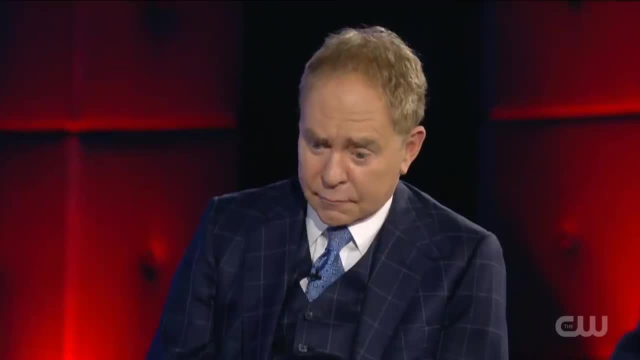 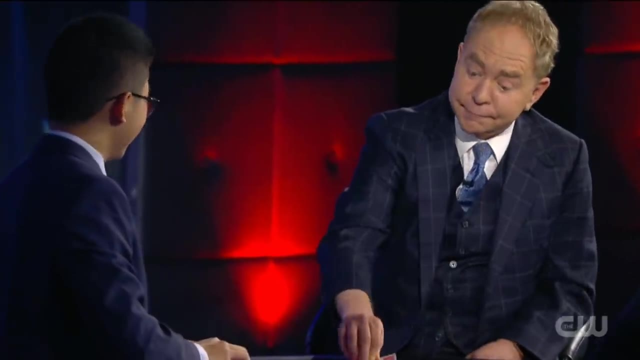 Exactly So. that means that Teller must have the three red cards. If you don't trust me, you can check again to make sure He doesn't trust me Here. help me mix the red cards into the black cards, just like this. 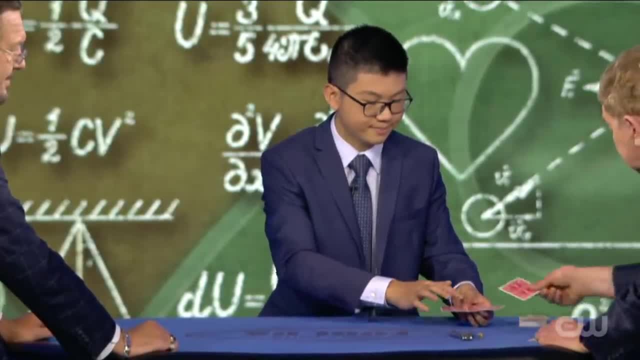 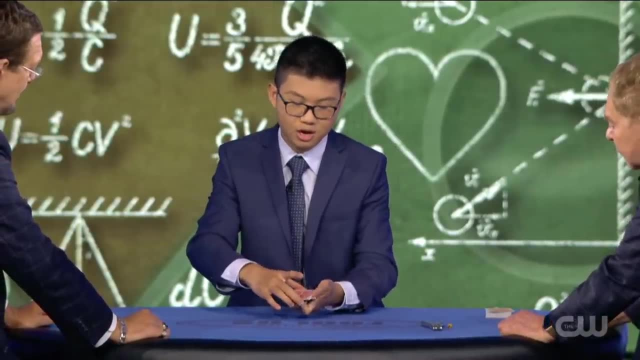 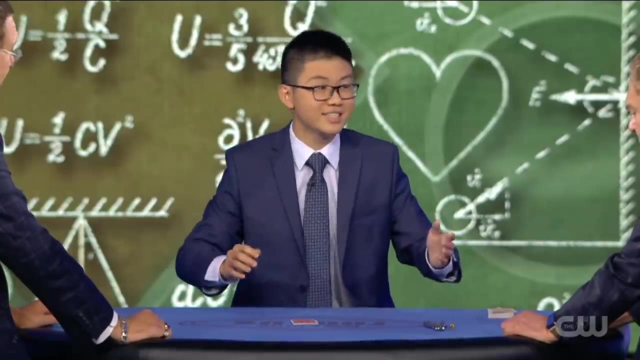 First one, Good And perfect. Now, once again, we're going to drop the cards and the black cards are going to pass through the red cards. I saw it. Did you see it, Pen Teller? I didn't. 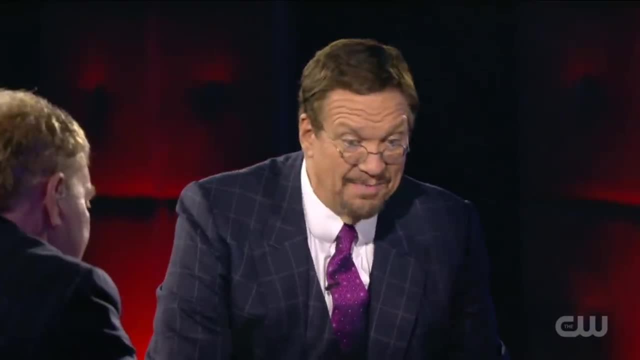 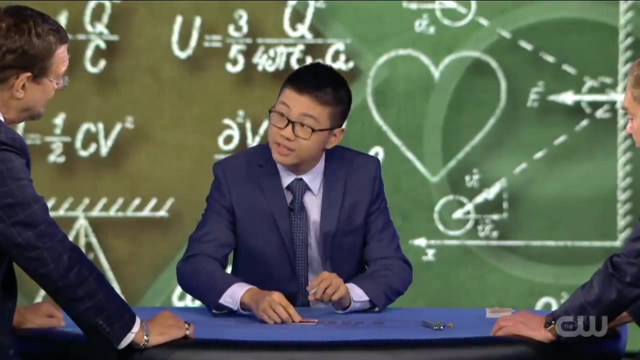 You didn't, I didn't. Come on, you're my independent observer. I didn't see them. actually, I just looked like you dropped them. Well, who knows, maybe it worked. Let's check it out. First card, that's red. 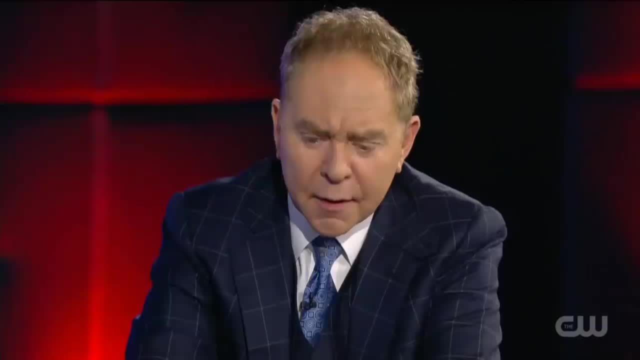 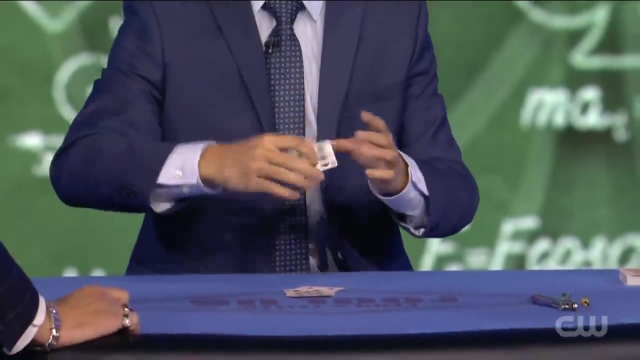 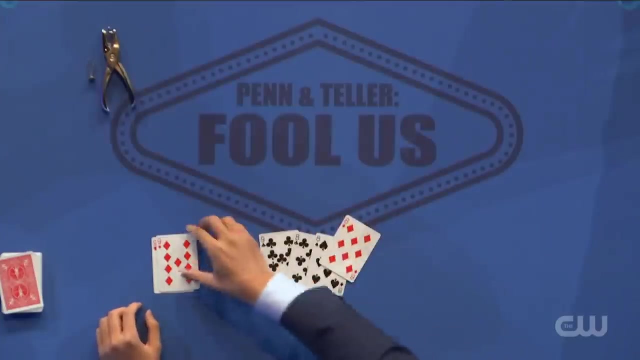 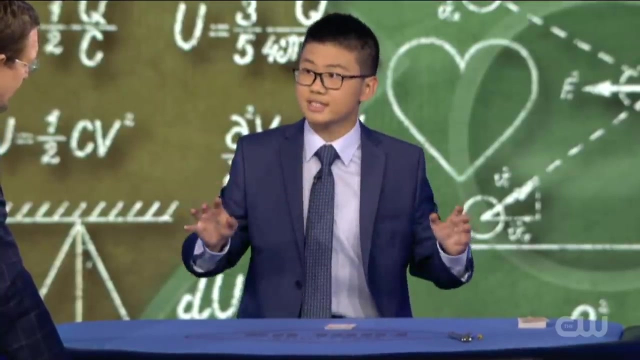 Red And red, Thank you, And over here, Thank you. I'll admit that, while this experiment appears to have been perfectly and scientifically fair, I did handle the cards after Teller mixed them, And as a magician physicist with incredibly fast fingers. 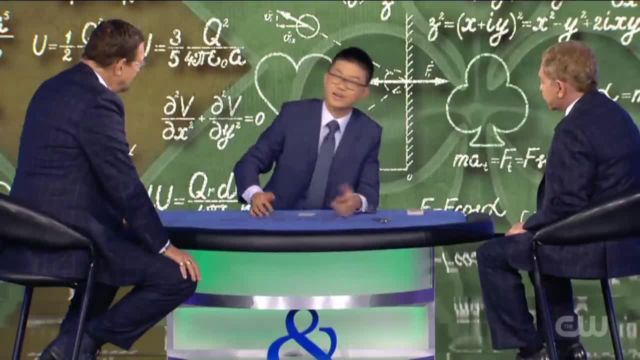 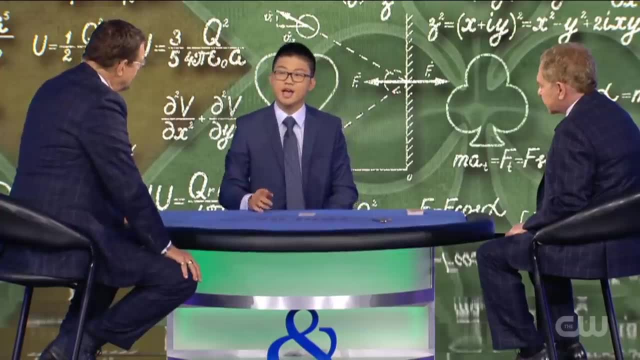 I might have done something. I might have used my hand, Who knows? So, for those of you who still may be thinking that this is a card trick and not a physics experiment, and to put all doubt to rest, I'm going to create a condition that only physics can solve. 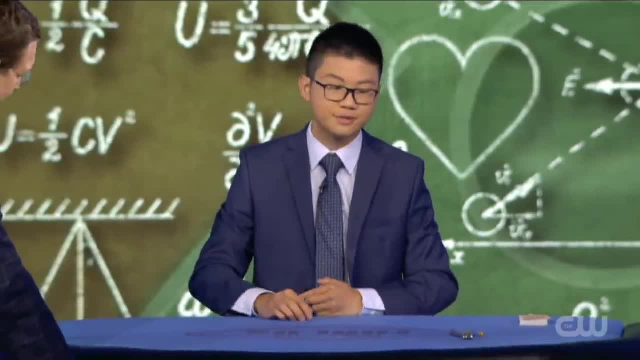 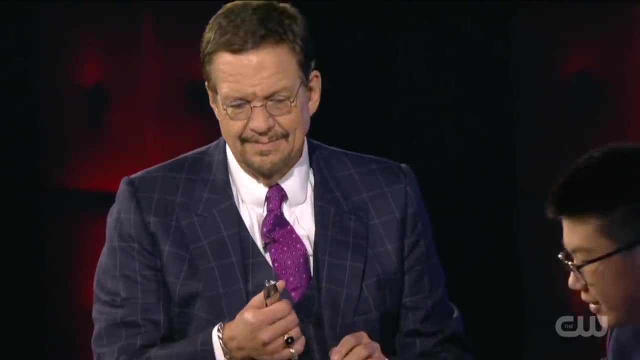 I have invented a sleight of hand prevention machine. The first part is this hole punch Pen- you can check that out- And the second part is the paper fastener. Okay Teller, you can take a look at that Now to prevent a sleight of hand. 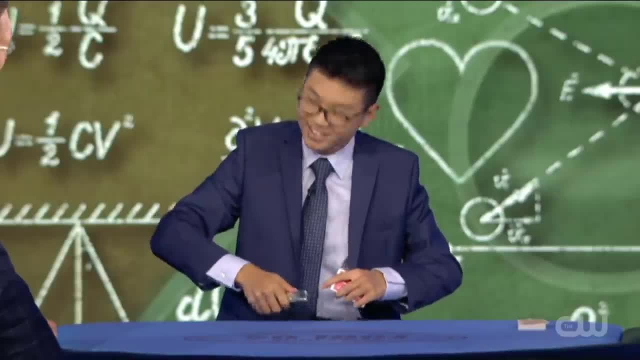 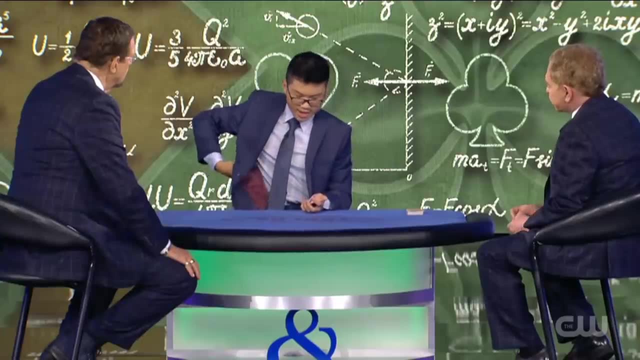 we just punch a hole in each one of my fingers, Just kidding. What we're actually going to do is punch a hole in the cards. There we go, That's good, And we're going to use that paper fastener. Thank you. 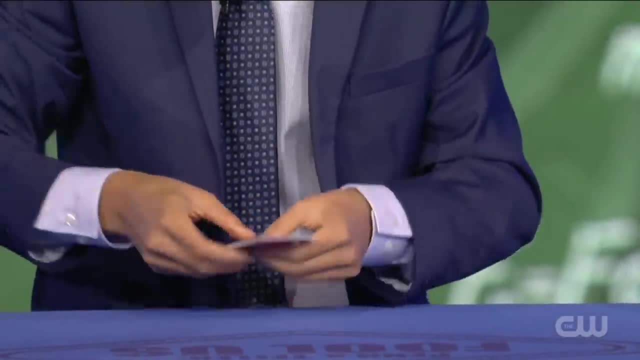 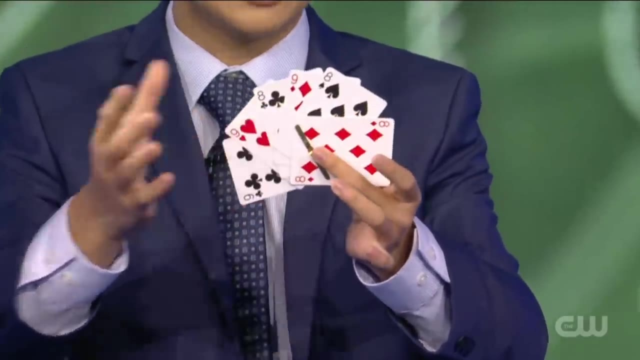 To make sure that we- I can't use sleight of hand to make the cards move Just like this. Now, if you take a look, the cards are really alternating- Red black, red black, red black- And you can see that there's no way we can change the order of the cards. 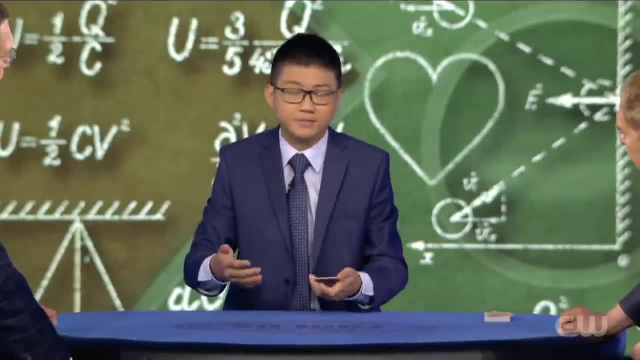 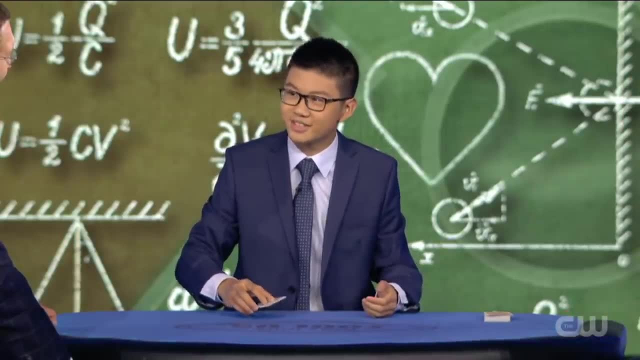 no matter which way we turn them, And if you think about it, if this were a card trick, the paper fastener will make it impossible. But this isn't a card trick, It's a physics experiment. I think that did it. 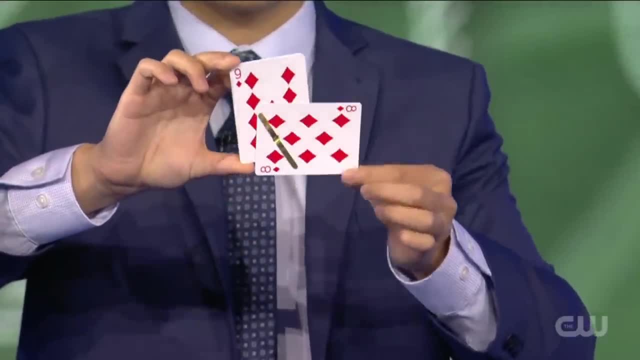 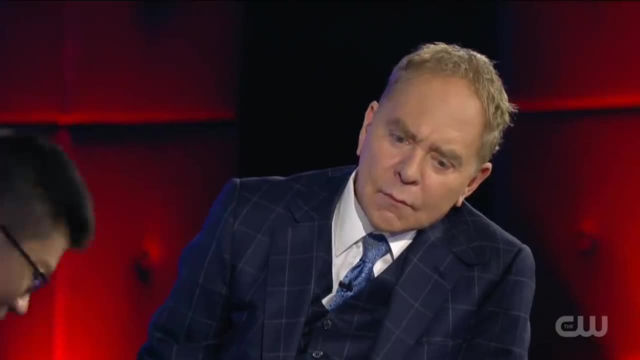 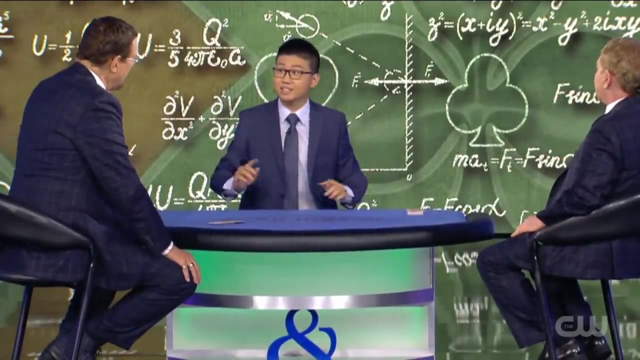 Look, That's red, Red And red And black, black and black. But that's all You see. the real physical evidence is in our control group. this stack of cards, Remember, it was totally mixed up before I set it down. 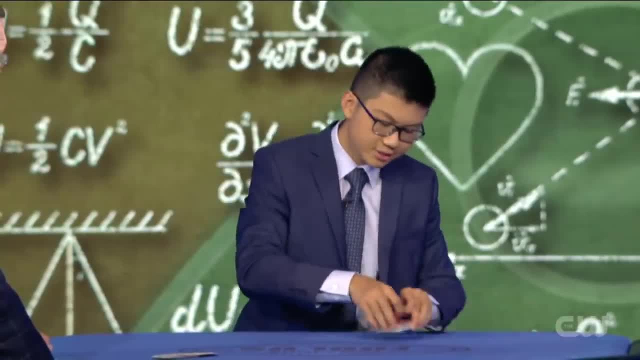 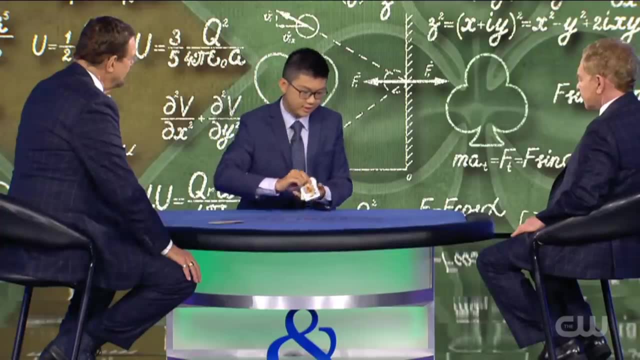 and hasn't been touched since. If black ink truly is heavier than red, this should prove it. And if you take a look, you'll see that all the red cards have come to the top and all the black cards to the bottom. 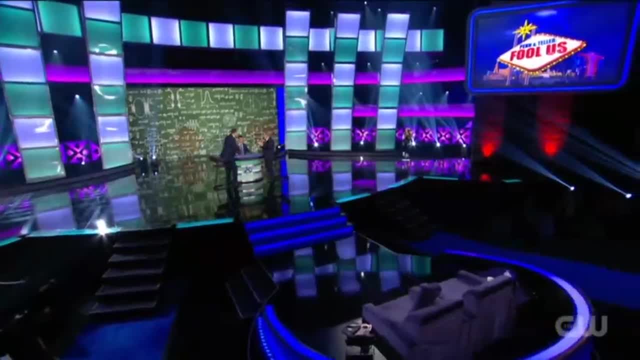 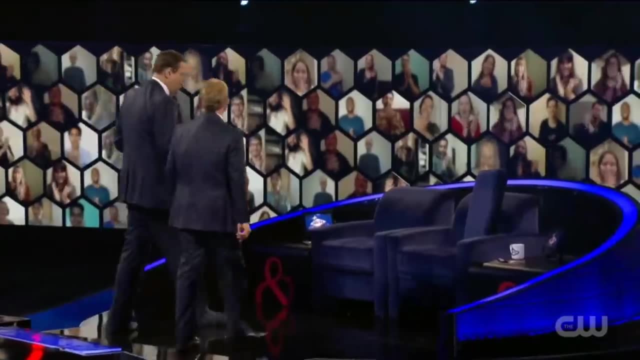 Thank you very much. Thank you Penn. Thank you Kelly. Can you take these wheels? Sure, Go ahead, Stanley Joe. Hi Hi, It's so nice to meet you. Yeah, nice to meet you, You're so incredible. 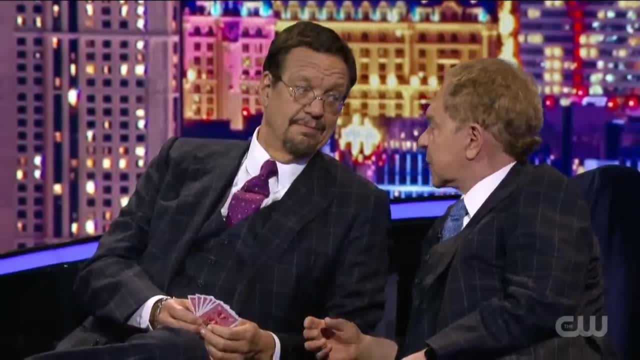 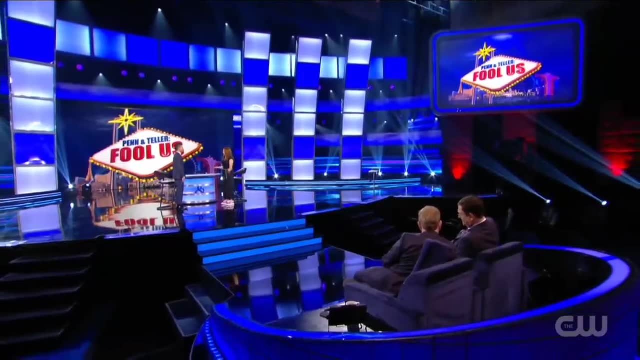 Thank you so much. How long have you been doing this Doing magic? Yeah, Only about three years. Wow, Yeah, Three years, and you're already here at Fool Us doing a close-up magic with Penn and Deller. Yes, 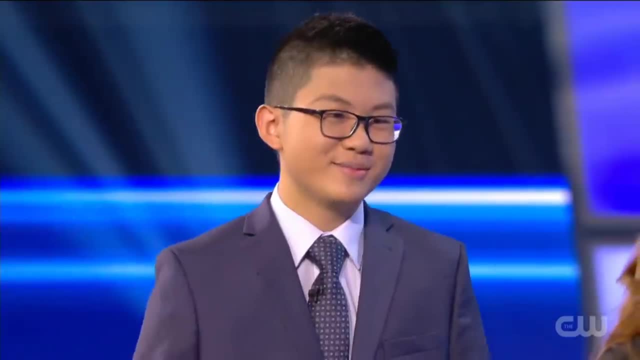 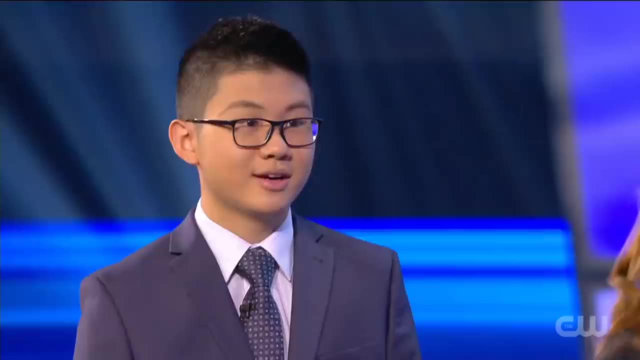 And is your family supportive? Yes, of course. Yeah, I wouldn't be here without them. That's true. It's so brave to do these tricks with Penn and Deller sitting right in front of you. Well, of course, I was nervous at first, but once I got out, 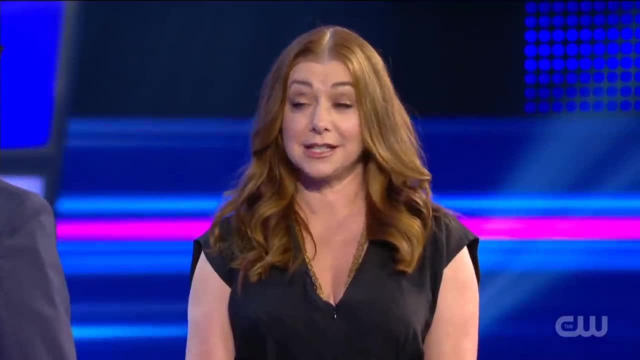 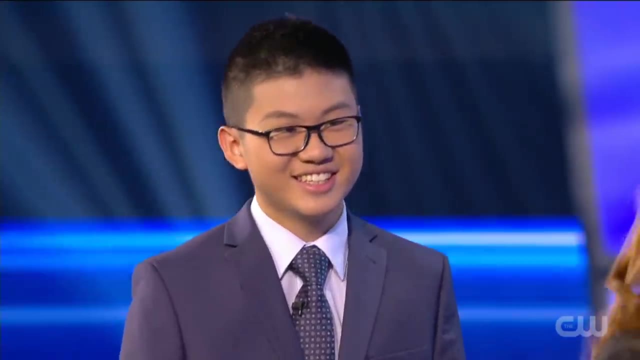 I just kind of got into the zone, And so are you actually good at physics as well. Yeah, I feel like you're good at everything. It's just a hunch. I don't know. actually. What other goals do you have for yourself? 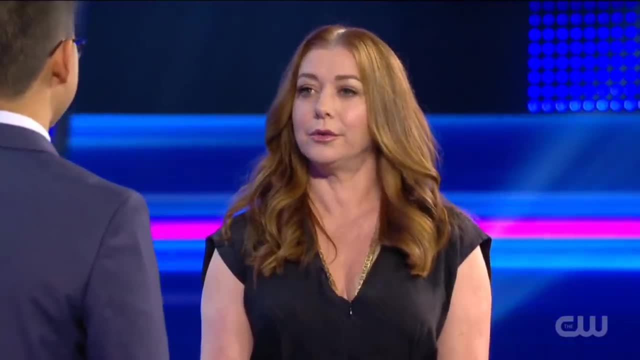 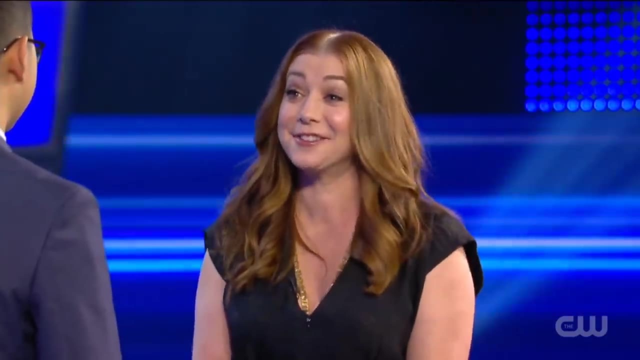 I really, really enjoy fencing. Ooh, It's just a really cool combination. It's just a combination of mental and physical skills. All right, Stanley, Let's see if Penn and Deller know how you did your trick. All right, 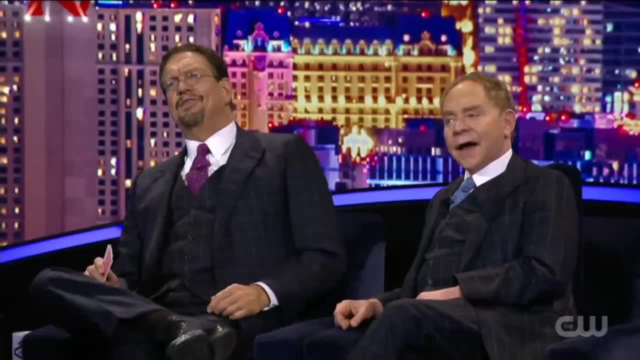 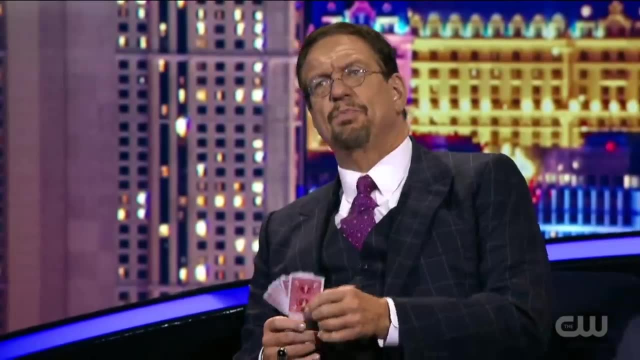 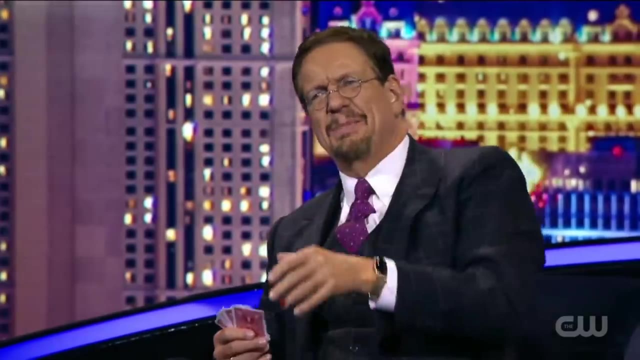 Stanley, Yes, I want to apologize to you because I think I cheated a little bit on the game. I asked you at the end if I could take this prop with me, and I'm really not supposed to do that. I mean, during this section I can ask about props. 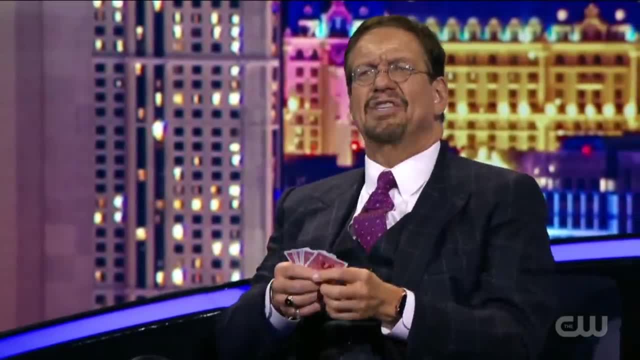 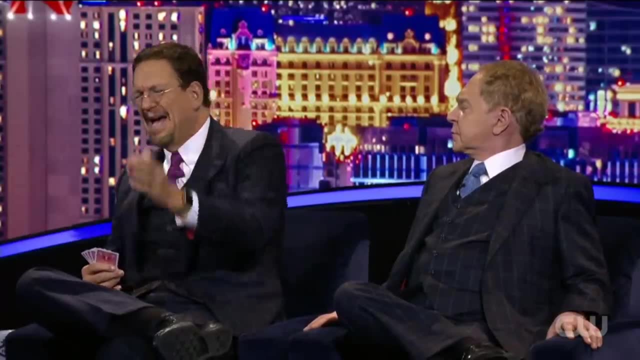 but I'm not supposed to, within the performance, ask you to grab something you didn't offer to me. And when I did it, my heart kind of sunk Because I said: here's this guy, 16 years old. He'd been in the country- what? three years. 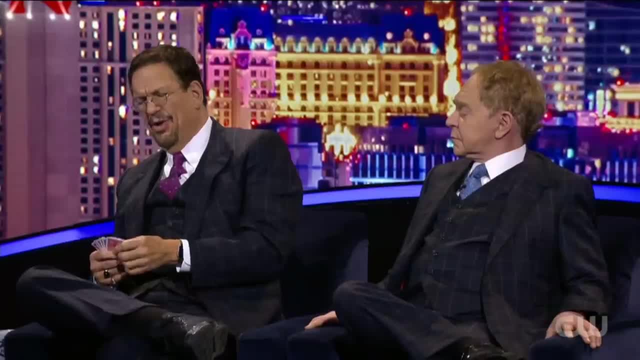 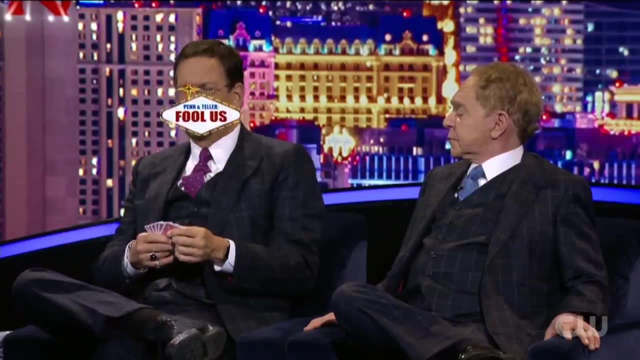 Three, four years, Four years, Four years Been in the country, four years learning English, learning magic. I'm here on our show and it was kind of a move to say: can I take this and put you on the spot? 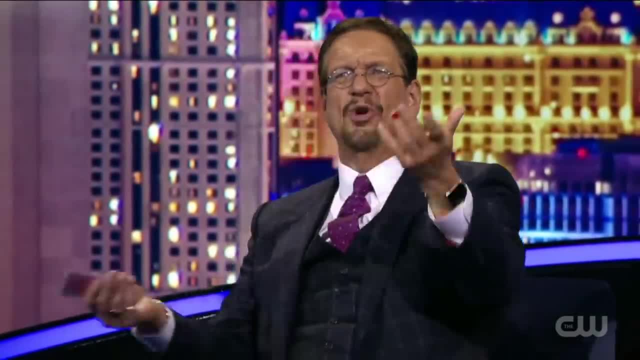 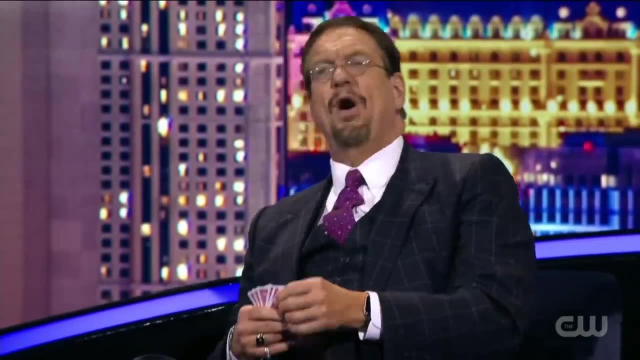 You don't have a choice. you can't say no, because that shows how the trick is done, so you have to say yes, then we take it away and we, we bust the trick. so i, i, i apologize, i don't feel like this is good or righteous, or i did.